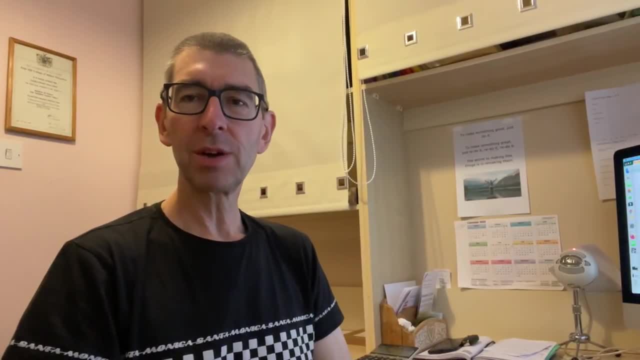 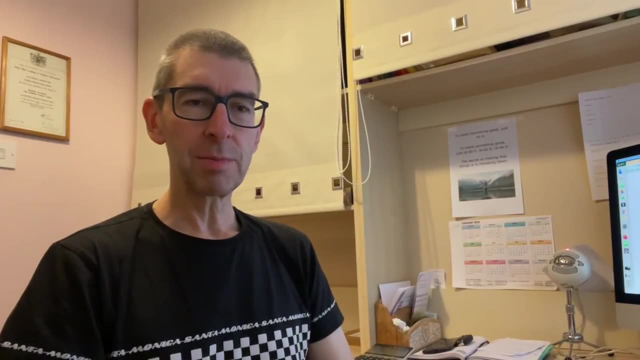 Okay, so we are in a place that we don't normally go. this is one of my offices- so what I want to do is just point out a couple of things first, just before we get into this. So, first of all, taxonomy in relation to orchids is very complicated and there are big, thick books written all about it. 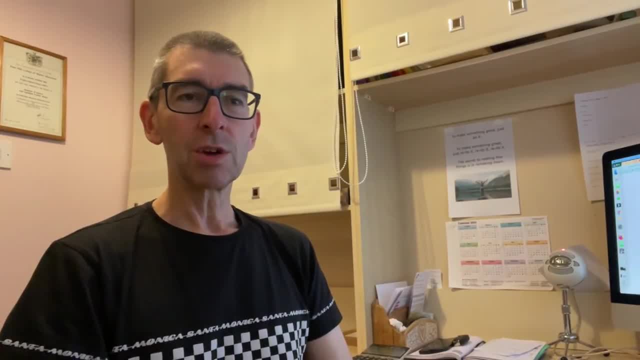 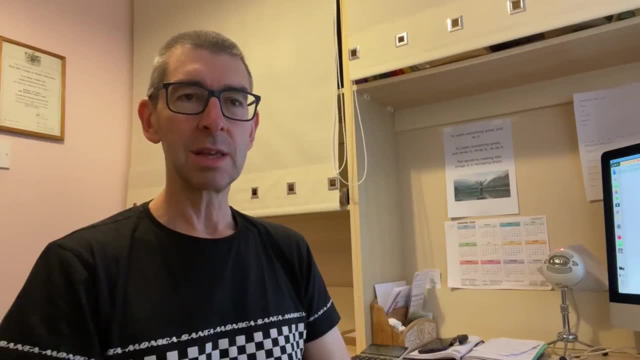 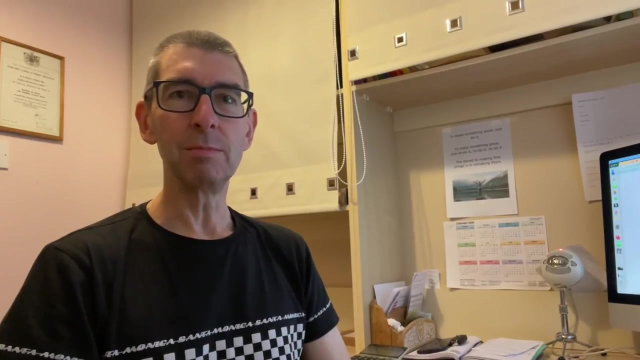 Now, as an orchid hobbyist, you've got to come to your own conclusion as to whether it's worth spending so much time on it. You know I've spent the amount of time that I've spent and I have to say I am a little bit embarrassed that I've not gone into this much earlier than I should. 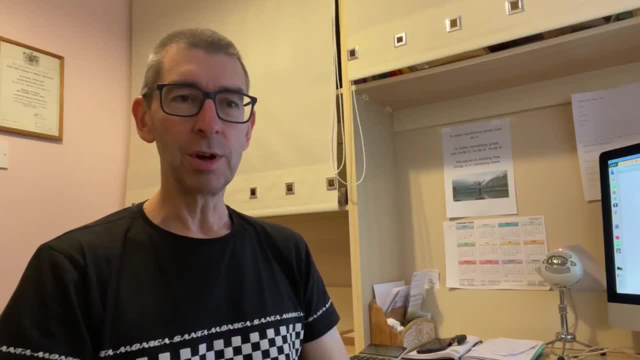 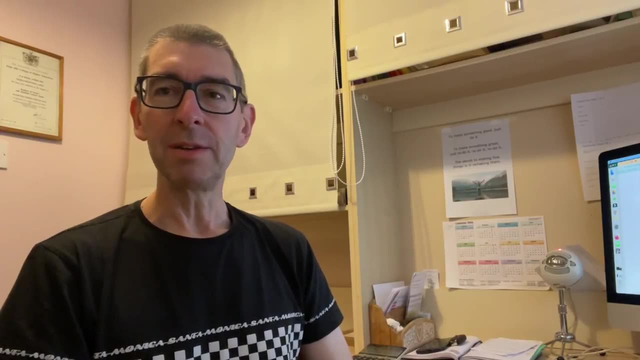 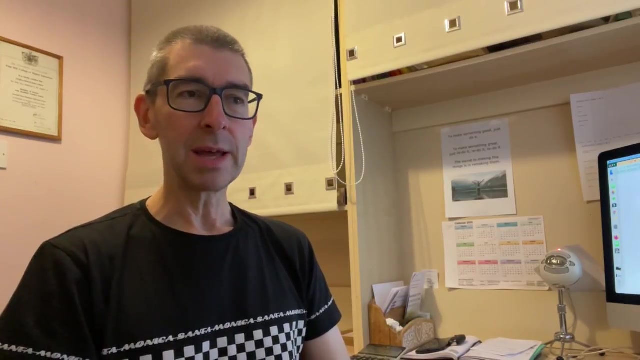 In the journey, as it were. however, this isn't my job. I have a full-time job and this is a hobby, and I don't get paid for it- well, not very much anyway, pence. So, having said all that, you've got to make your own mind up and this way, may well be common knowledge to lots of orchid enthusiasts. 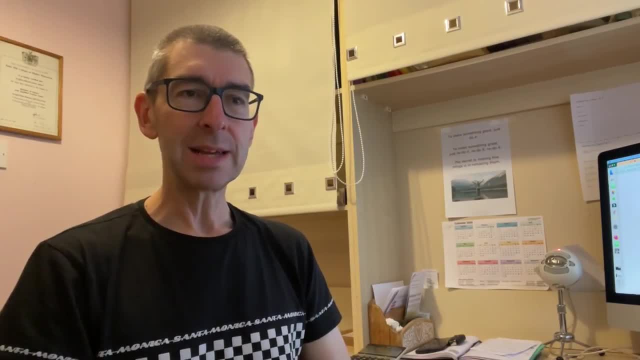 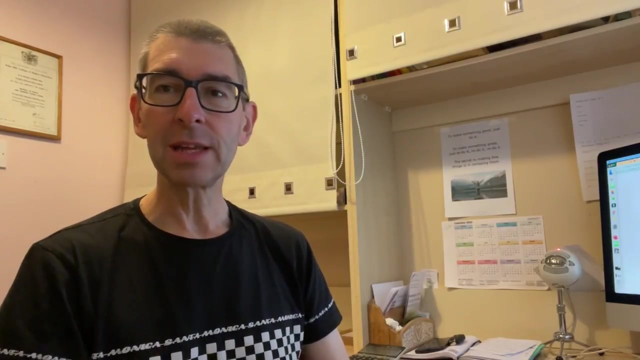 but it wasn't for me. so I have done my best to fill those gaps and try and come up with a solution, The solution that works for me, and I'm really hoping this will enable me to take my hobby to the next level, and if you find it useful, then obviously that is even better too. So I don't 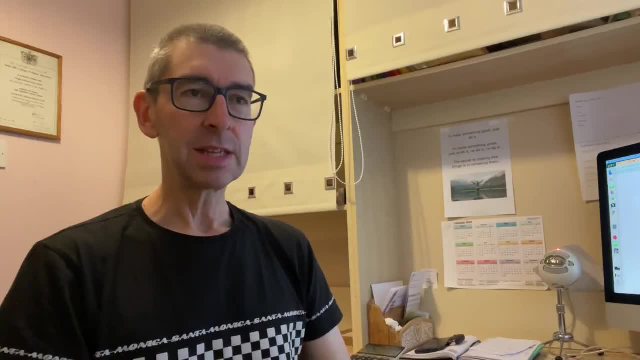 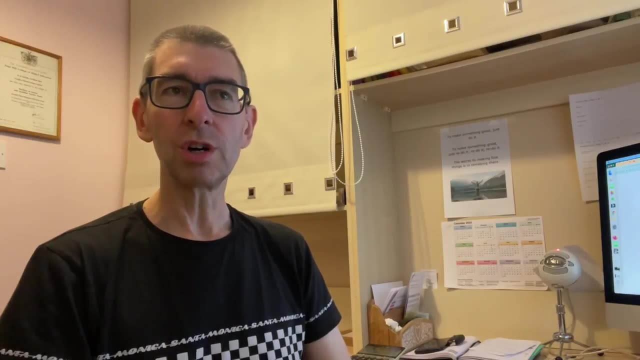 understand it all. let's make that absolutely clear. this is the understanding that I've got so far after spending a couple of days reading loads and loads of sources. There isn't one source that completely explains everything- not to my satisfaction anyway. I found that it was better. 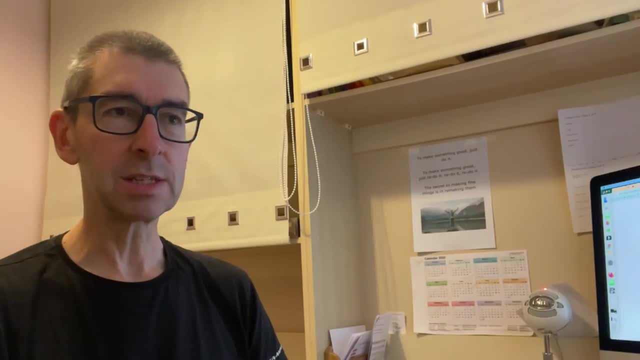 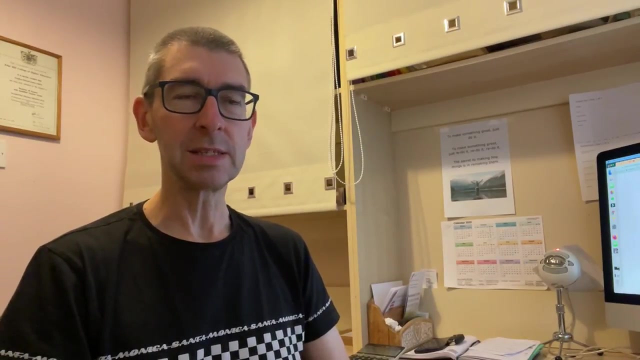 to read various sources. There's some good stuff on the American Orchid Society. There's some good stuff on the Atlanta Orchid Society. I did come up with a few other different things. I think First Rays had some good stuff. I'll put some links in the description of some various places that you can get information. 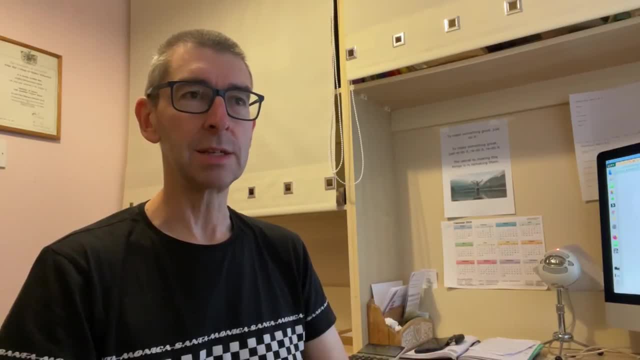 on this. There is a really good website that Terry at TD- more than just orchids- pointed out, that you can actually do a search for hybrids and it gives you the names of the parents and the care needs and so on, And you can also do that on the Royal Horticultural Society. 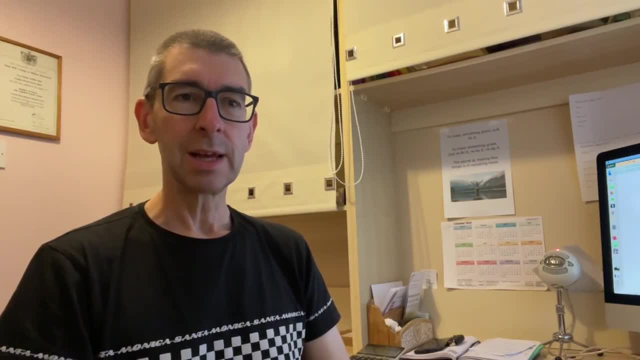 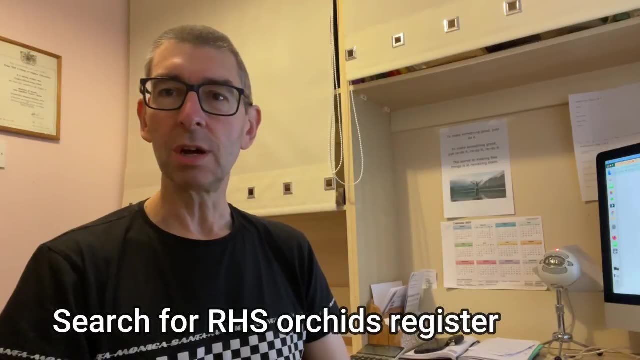 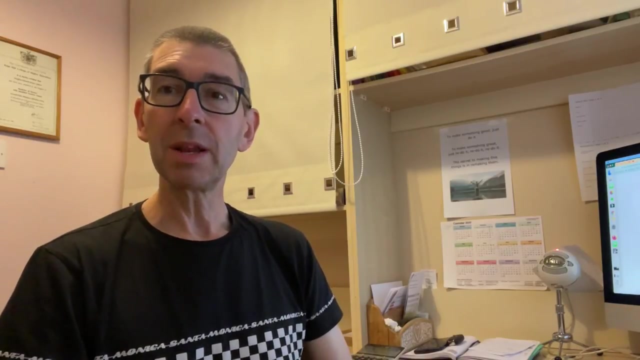 website as well, which allows you to search for hybrids. It doesn't give you as much information, unfortunately, but they are the official worldwide register of orchid hybrids. Okay, so I think we've covered everything there. If you are someone who is already familiar with this, 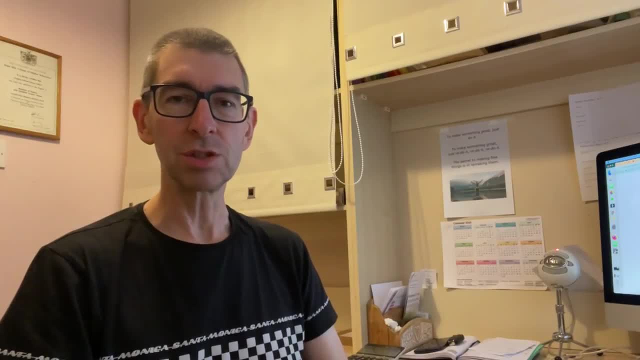 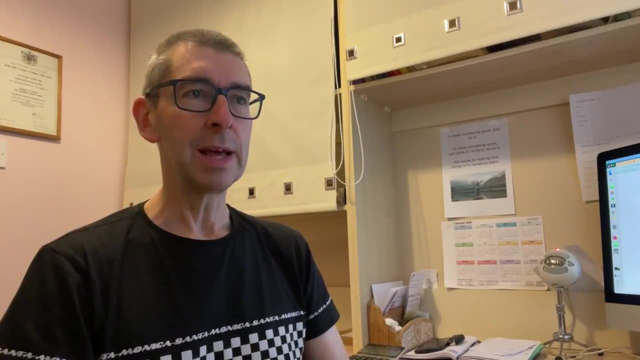 stuff and I know there are people who comment regularly who are already familiar with this stuff. then please do point out any glaring errors. Not that you need telling about that. I'm sure there may be some errors, so point that out to me and if you can help to move. 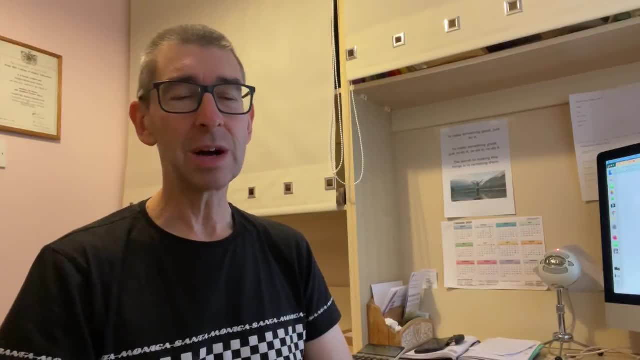 the discussion on again. put that in the comments And if you find it useful, that would be great for people to point that out, or give me a like, or put that in the comments as well. So, having said that, what I'm going to do is I'm going to write it out for you what I understand. 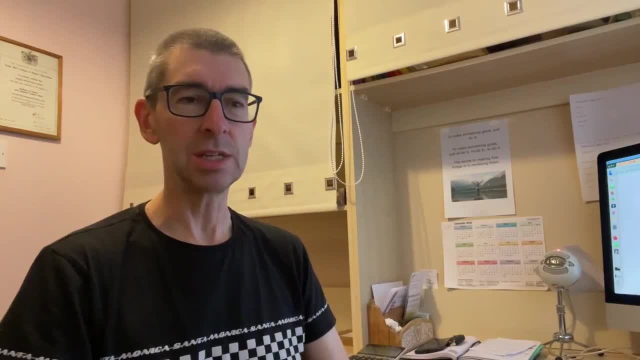 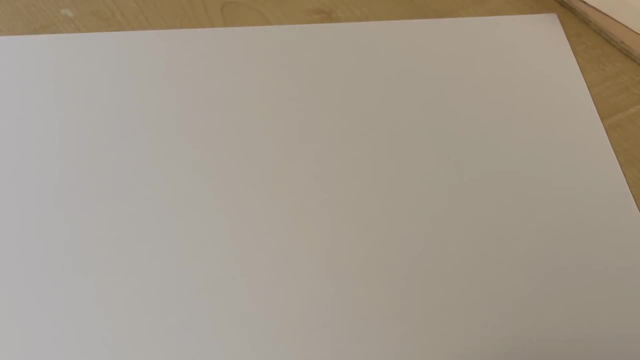 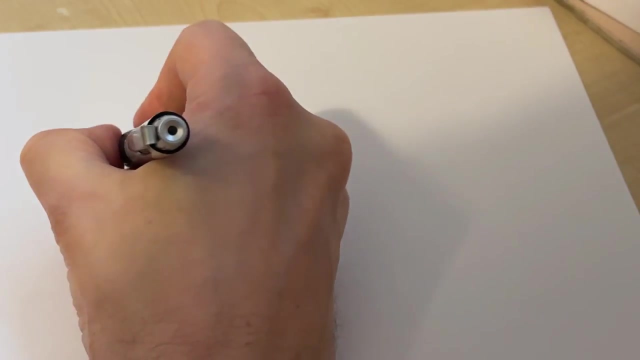 it in like a bit of a concept map. I'm going to start with species, so let's jump into that. Okay, I hope you can see that. So, first of all, orchid naming Is split up into two rough groups, So we're talking first of all about species, orchids. 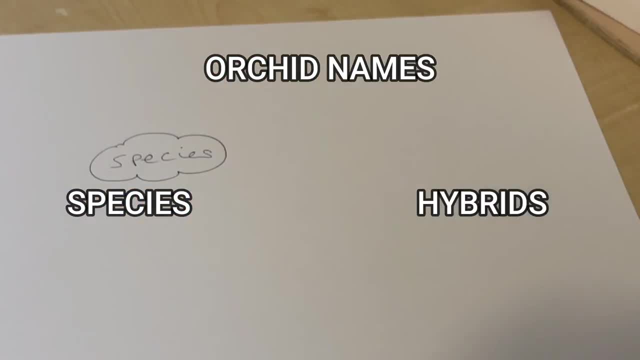 So I'm going to put that on my paper there. And species- orchids are those that you find naturally in the wild, So a couple of examples might be a Dendrobium kingianum. So I'm going to write that down and I'm going to abbreviate that, just because that's something else. that's. 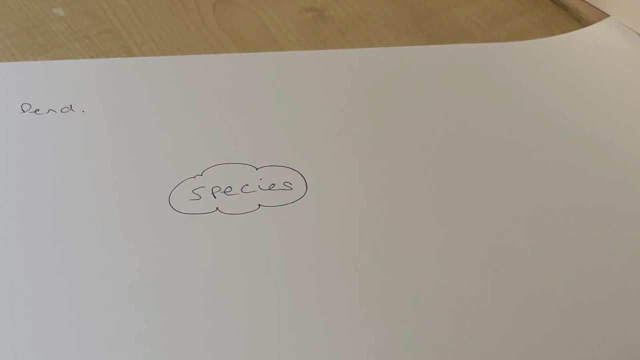 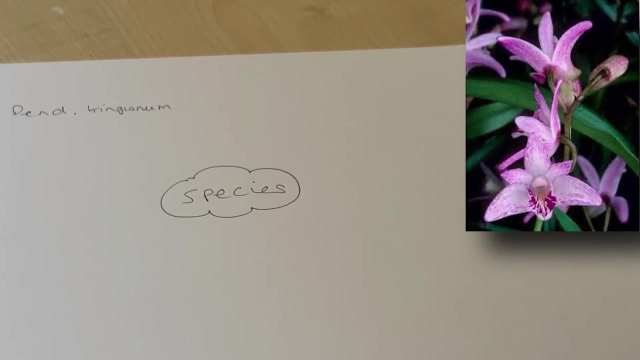 worth pointing out. I'll have to move that over a little bit. So Dendrobium kingianum. Now, this is where it gets a little bit confusing because, unfortunately, and I'm as much to blame as anybody else- When you write labels out, when I write them out, when sellers, people, 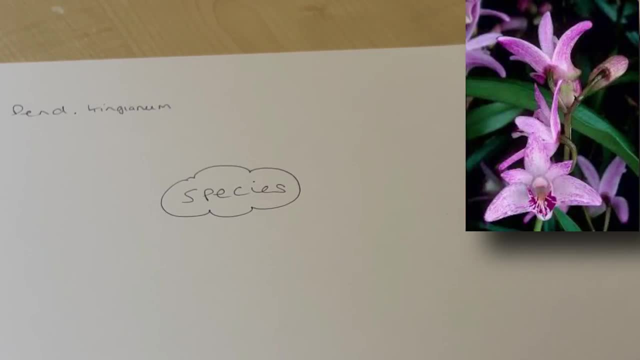 on eBay, people in garden centres and other people who sell orchids. when they write them out, they are not familiar with orchid nomenclature, So they will simply copy what they see, or they will mix up capital letters, Lowercase letters And, as I've since found out, those things matter, And this is where 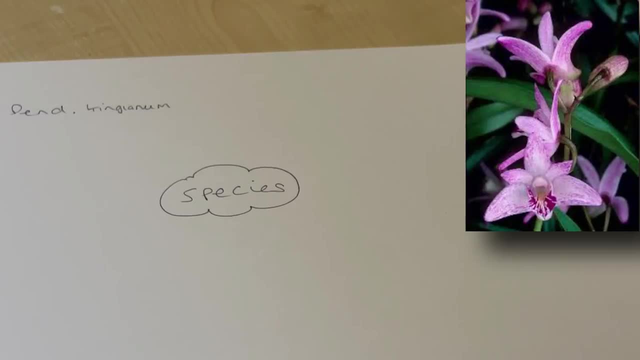 it gets a little tricky. Also, I cannot write in italics, and that also matters. So the first thing to point out is that if you see an orchid which has a name like a Dendrobium kingianum- and it is all in italics, So I'm going to point that out there- It's all got to be in. 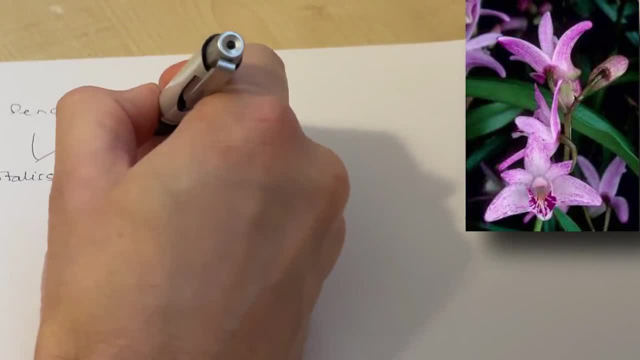 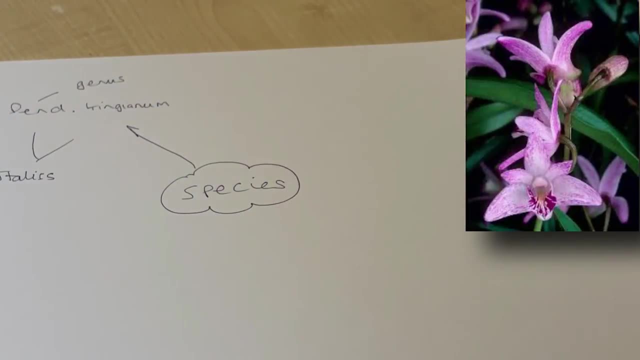 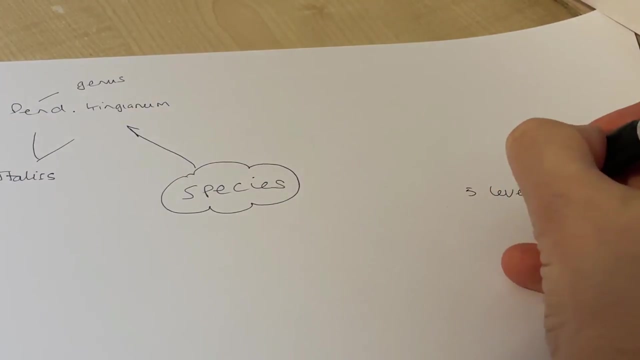 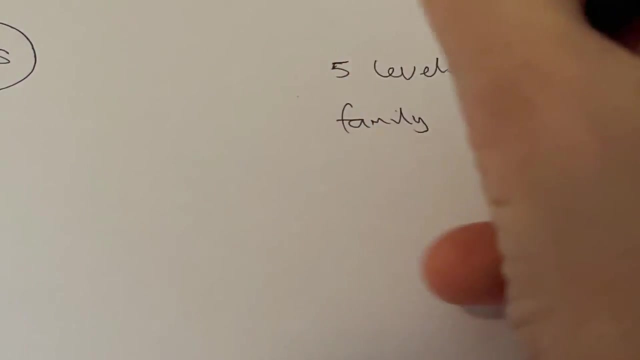 italics. That tells you that that is a species, orchid. okay, Over here we have the genus. Now this comes from the general plant family group. So there are like five levels of plant groups, plant groupings, until you get to family We're. 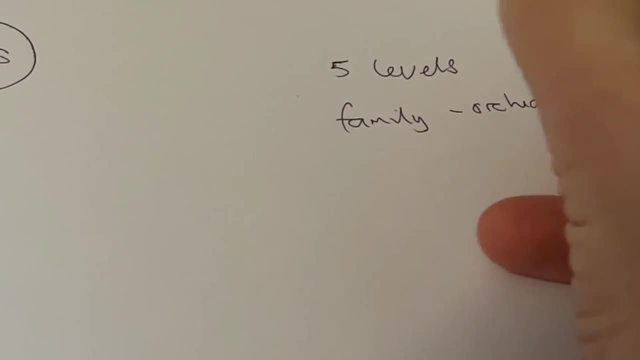 obviously dealing with orchidaceae, Okay, Okay. So underneath orchidaceae- the next level down- then we have the genus, then we have the species and, of course, the hybrids as well. So orchidaceae family genus are things that people are very familiar with in the orchid. 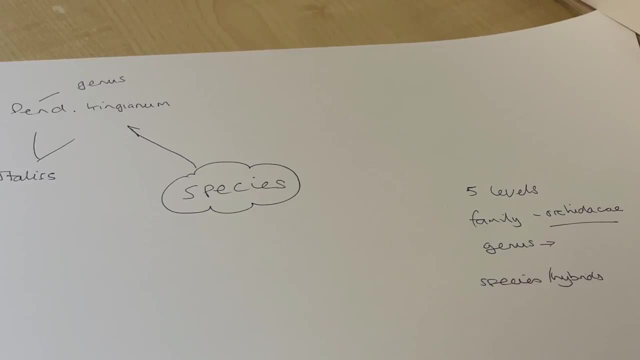 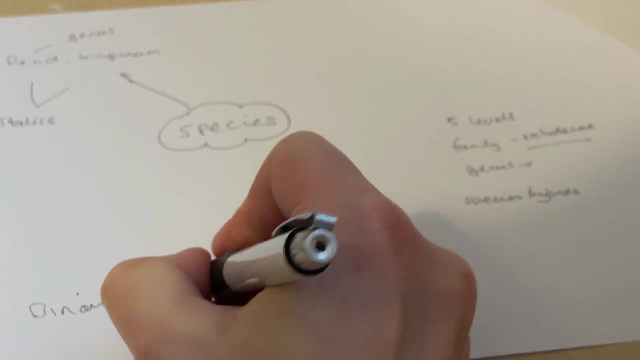 world. So words like Phalaenopsis, Catlea, Dendrobium, Mastivalia, all those kinds of things. they are the genus, Okay, So what we're talking about here, this is the binomial naming system, and it was devised. 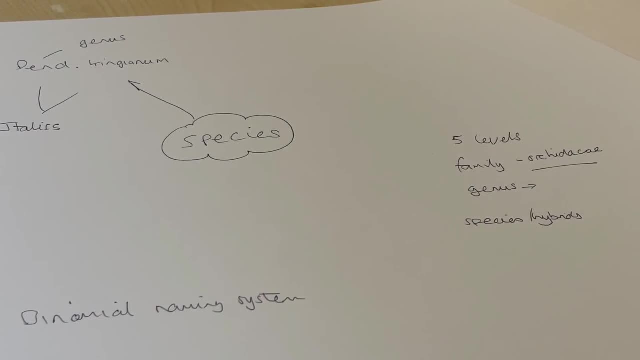 by a man called Carl Linnaeus in the 18th century. Now Carl Linnaeus seems to be arguably like the father of orchid naming, because he came up with this system and prior to this it was very, very mixed up and confused, You could. 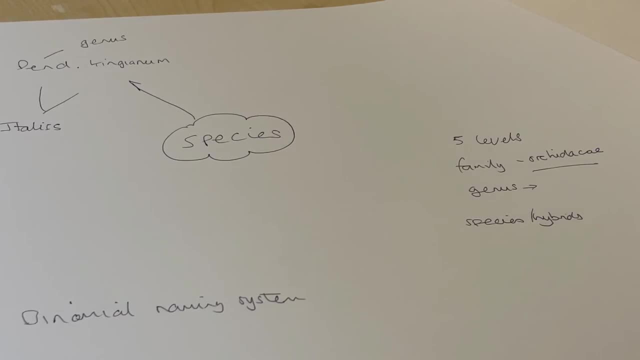 say that it's still mixed up and confused to some degree. Okay, But if everybody could follow all the rules, then it wouldn't be. This is where the modern tendency to abbreviate everything and not really take much notice of these things will no doubt cause even more confusion in the future. 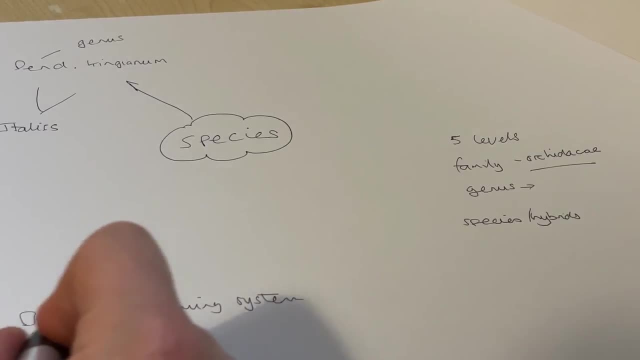 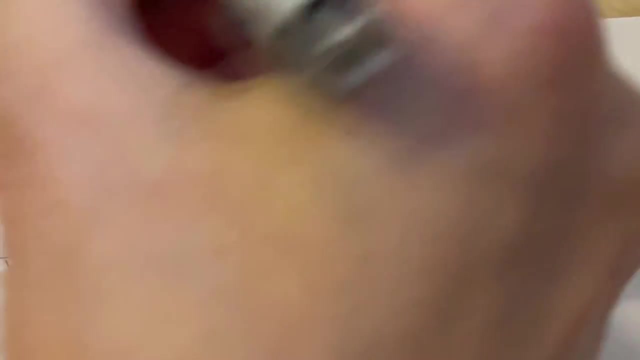 So this is the binomial naming system. Binomial means two names, just like me and you two names. So we're talking about Dendrobium kingianum. We've said, if it's all in italics, If the first letter of the genus is a capital letter and if the first letter of the species 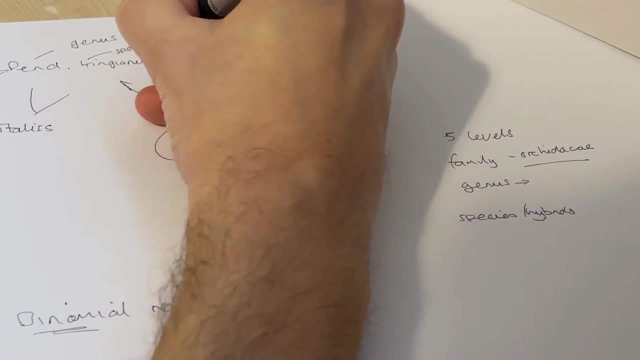 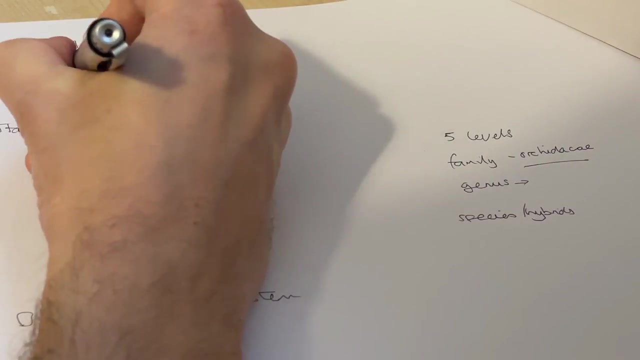 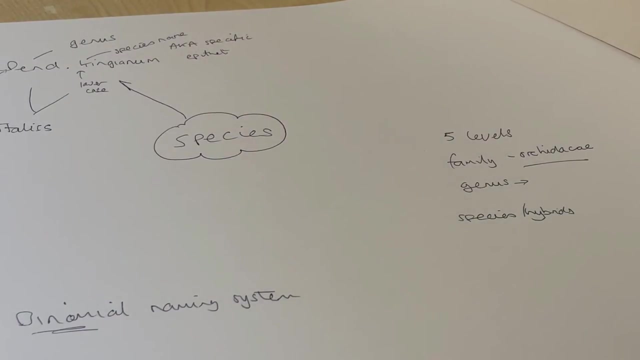 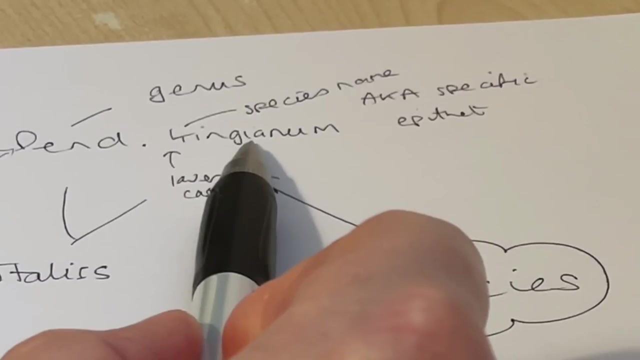 name and that's the species name, also sometimes known as the specific epithet. If that has a lowercase letter, then you know that that orchid is a species orchid. So if you've got two names- genus first, species name second, also known as specific epithet- 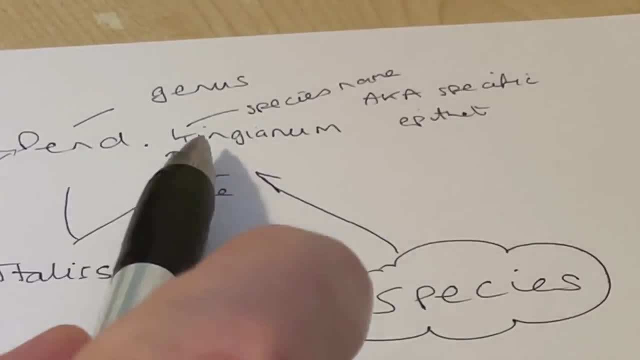 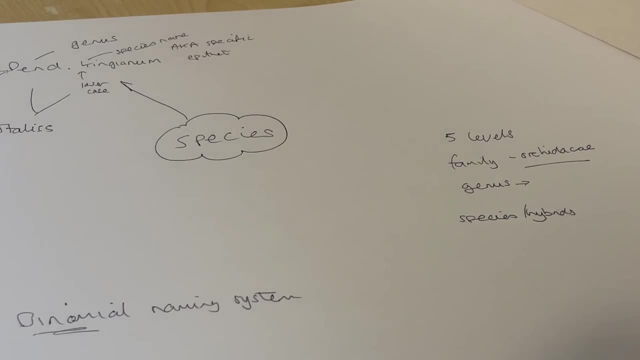 all in italics, both words: capital letter on the genus name, lowercase letter on the species name. then you know it's a species. Okay, You can see how it can easily get confused. There's a lot of things to remember, although having just done a little bit of practice. 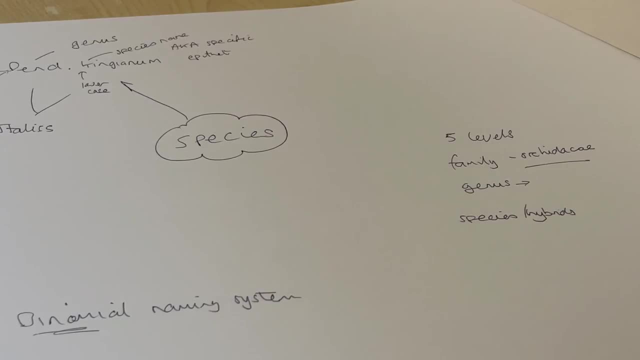 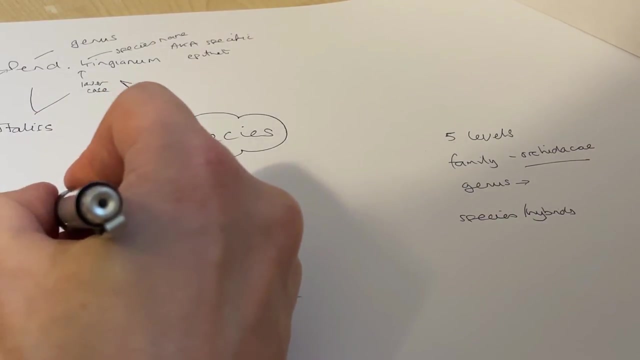 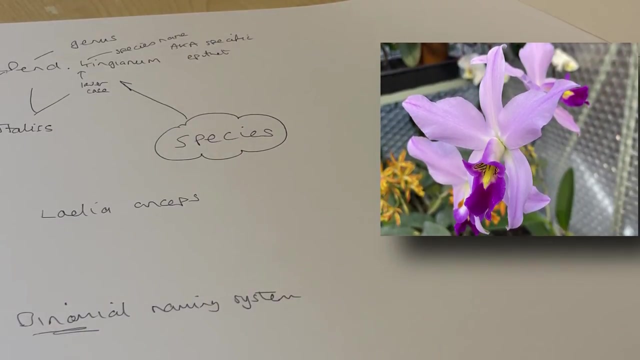 with some of my own orchids it very quickly gets quite easy. So after those labels That I took, these are the ones that were species. So we have Lelia Anseps. So if I could write in italics that would all be italics. 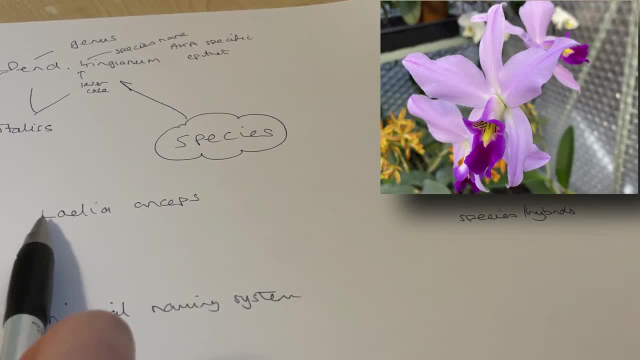 Genus name, species name or specific epithet. Genus name begins with a capital letter. Species name begins with a lowercase letter. Of course it would be all italics, as I've just mentioned. quite straightforward, really. And just as an aside, 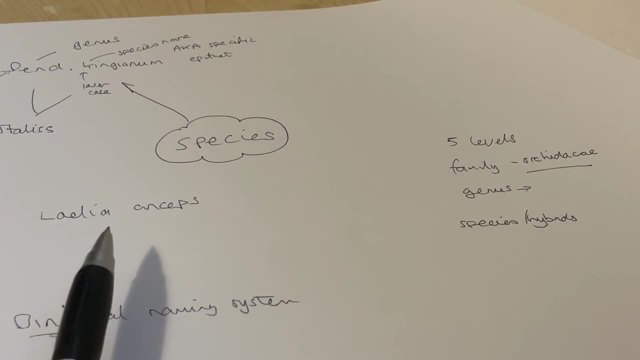 These genus groups Were originally based on morphology, and morphology is simply how various plants could be grouped based on the characteristics of that plant. So you might've got a few plants that had similar blooms or similar numbers of petals or similar ways of seed dispersal or similar growth habits, and so on and so forth. 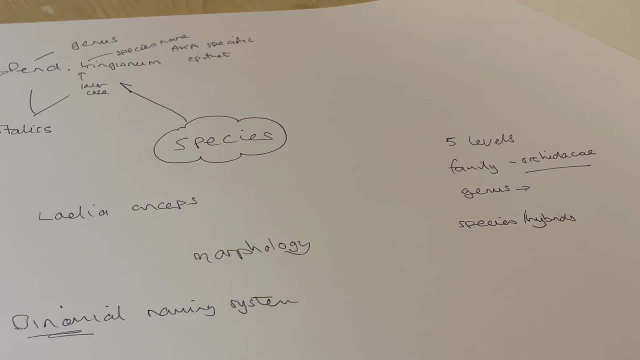 And it was that morphology That originally helped to decide on which particular genus an orchid went into. Now, as time has gone on and science has progressed- Some people might say regressed, if they are not particularly happy about a change of a name. 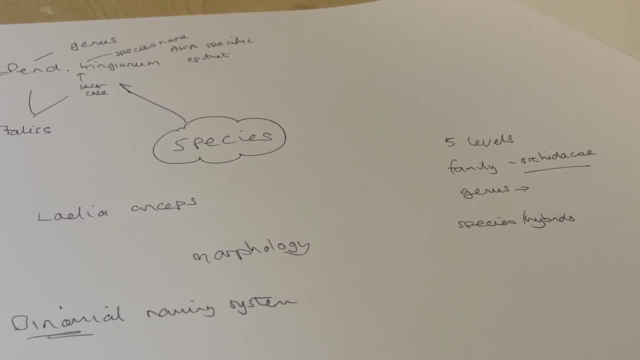 But as time has gone on, science has started to use other methods to decide which branch of the evolutionary tree an orchid comes from, And in many cases that's led to a reclassification, So that some of those orchids have been put into other groups. 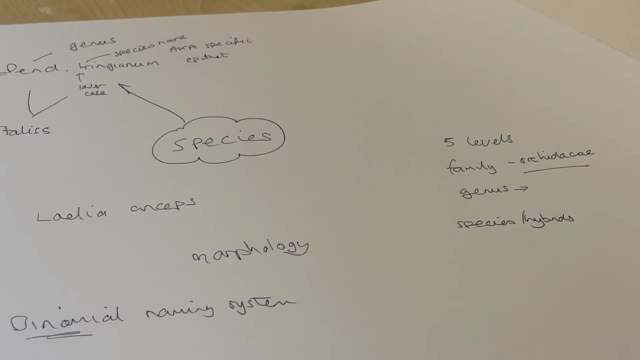 So an orchid that might have been in one genus then gets moved into another genus. One example that I can give- and it's not actually an orchid, but it's just one that springs to mind because it's in my greenhouse- Is that I have a Mandevilla. 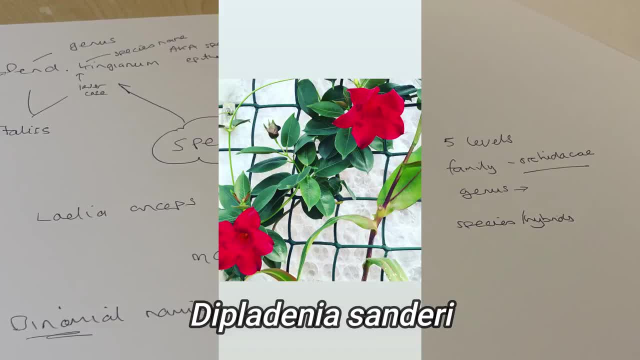 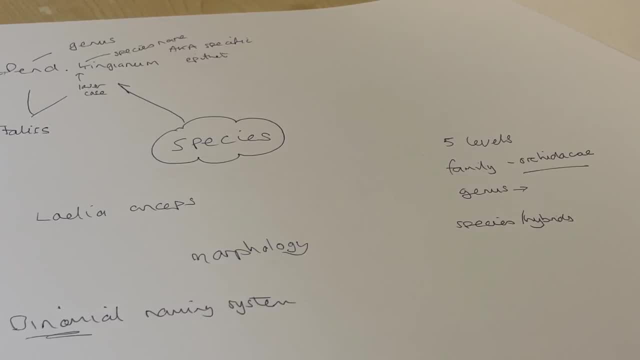 Now it was originally labeled for me a Diplodinia sanderi. Sanderi is the species, Diplodinia was the genus. However, the genus Diplodinia got lumped into Mandevilla, So there is no more genus called Diplodinia. 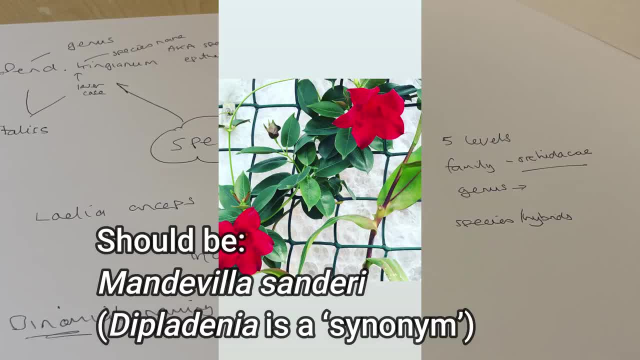 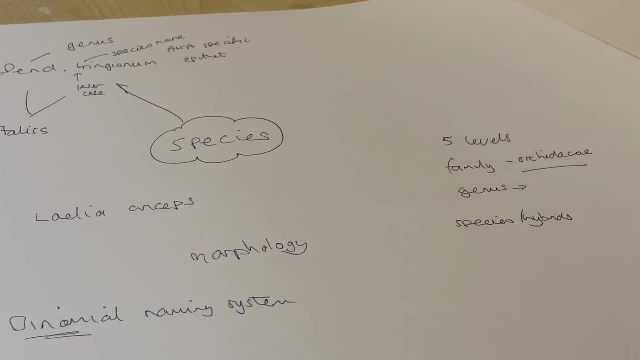 But unfortunately that Diplodinia has continued and people have continued to use that because that's what it was originally labeled as. So we then say that that is a synonym, And you'll find that there are lots and lots of orchids that have these synonyms because they've had various name changes over the years. 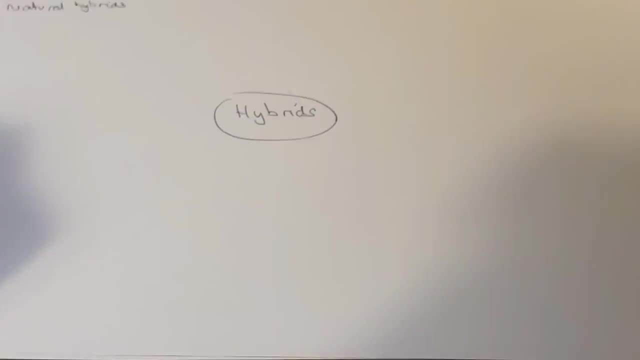 OK, we're going to start with natural hybrids. So natural hybrids are when Two species get together in the wild and create a third plant. So one example of that. again, we'll stick to the Dendrobium kingianum. 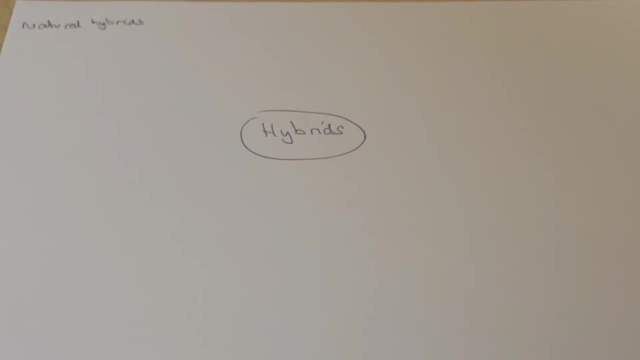 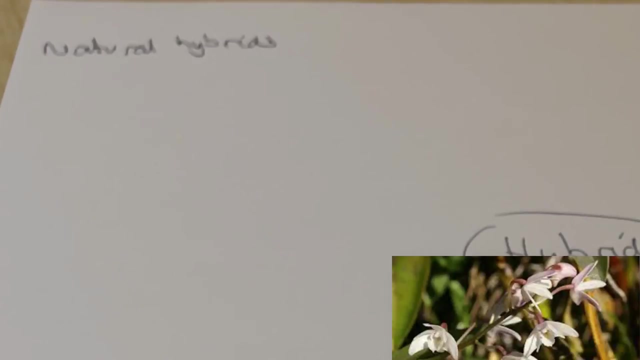 Well, that's what we were talking about before. So a natural hybrid of that is Delicatum. Now I was given a Delicatum and it's actually been labeled incorrectly. So Dendrobium Delicatum should look like this: 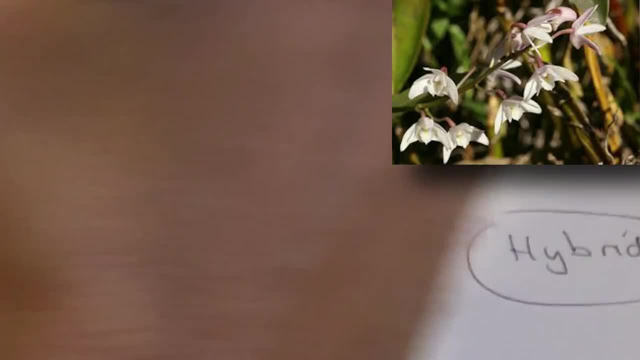 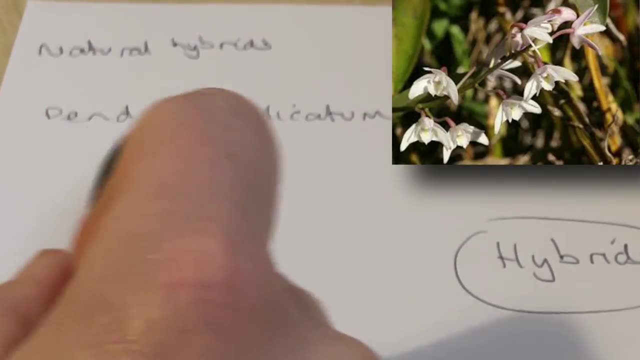 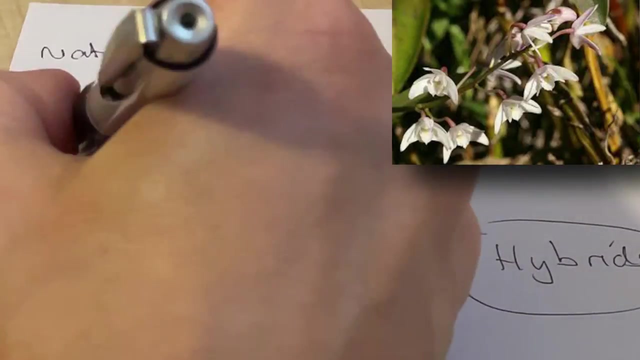 And again I'm going to abbreviate it just to save a bit of time. It should have a cross in there. The same rules apply that we had before, So all that should be in italics. I do believe that the cross shouldn't be in italics, although I did see a bit of information that said it should. 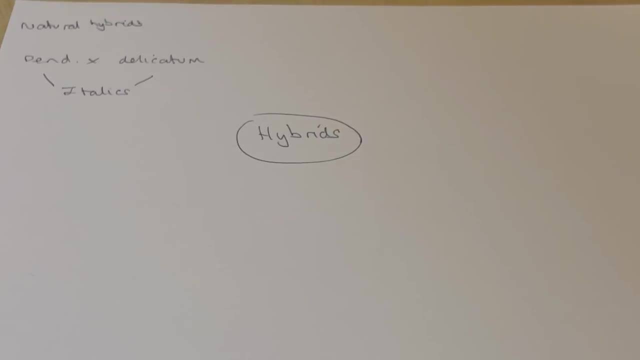 So I'm wondering whether there are slightly different systems depending on which side of the world that you're in. So let's just say, from the information I read, all in italics except the cross. So it's a Dendrobium Cross Delicatum. 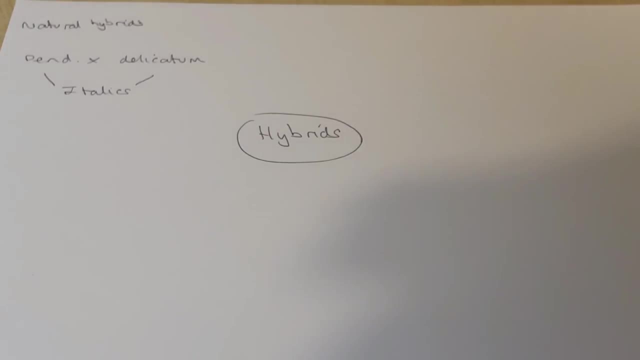 And that's a natural hybrid between Dendrobium Dendrobium Kingianum and Dendrobium Taberae. So in the wild those two natural species will get together and produce this natural hybrid. Now you might see that written slightly differently. 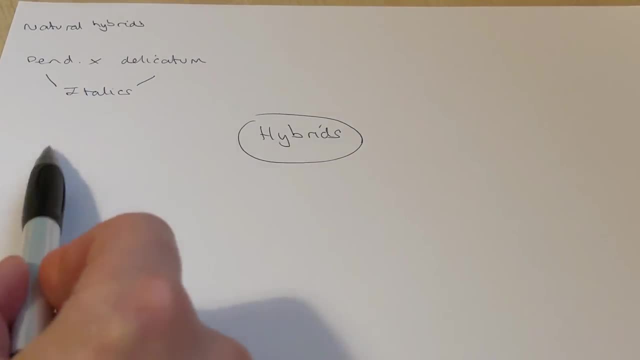 I'm not going to write it out, but you might see it written: Dendrobium and then in brackets the two species that are crossed. So it would actually look like Dendrobium and then in brackets Kingianum crossed with. that's the cross in the middle Taberae and close your brackets. 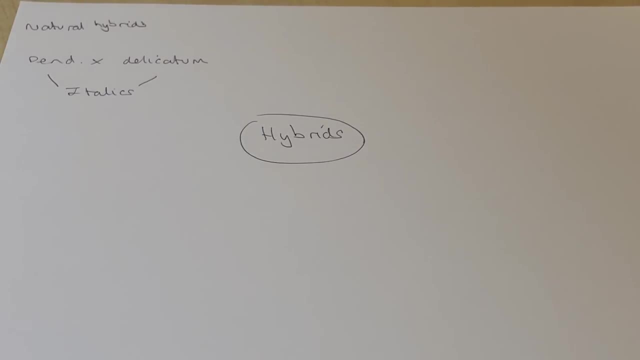 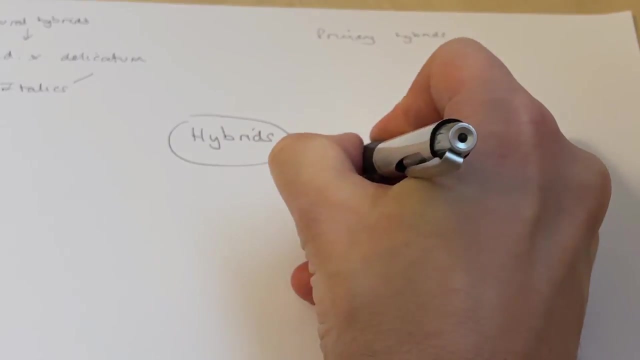 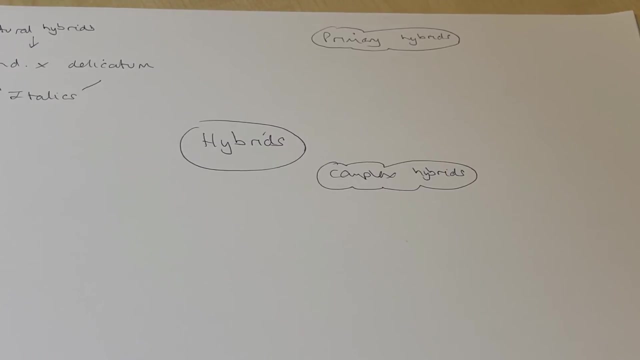 So that will also be in italics. So this is where things get a little more complicated. So we're talking about hybrids now. We've said that's the natural hybrid, but we can also have primary hybrids and complex hybrids. OK, so a primary hybrid is similar to a natural hybrid in that it's two species that are crossed together. 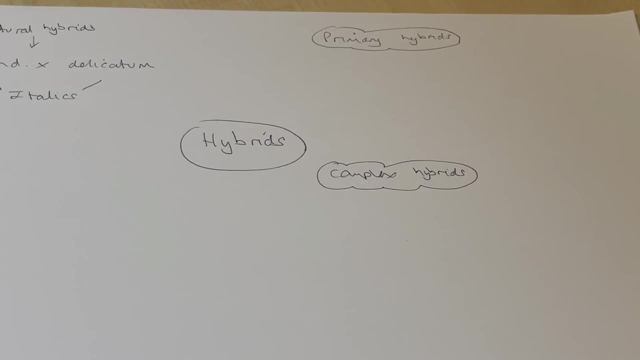 However, these do not occur naturally in the wild. So you might have One species from one side of the world and another species from another side of the world, and they don't ever come into contact. That will be a primary hybrid, sometimes called a primary cross. 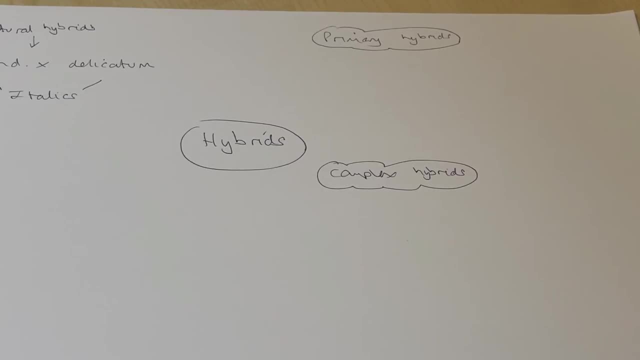 So let's have a look at how one of those might be written out. Now, I can't actually use one of my own, mainly for the fact that I don't know if they're primary cross or not. What I have to do is go through them all, look up the information and find out whether they are actually primary crosses or not. 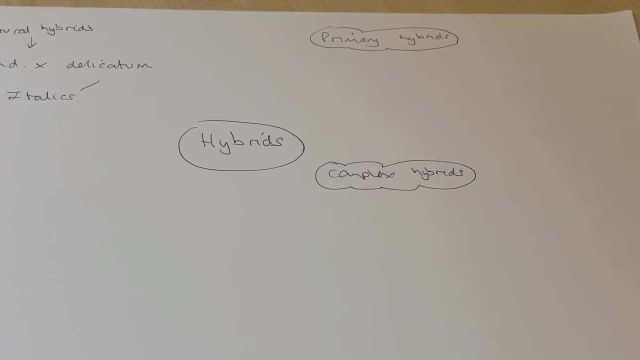 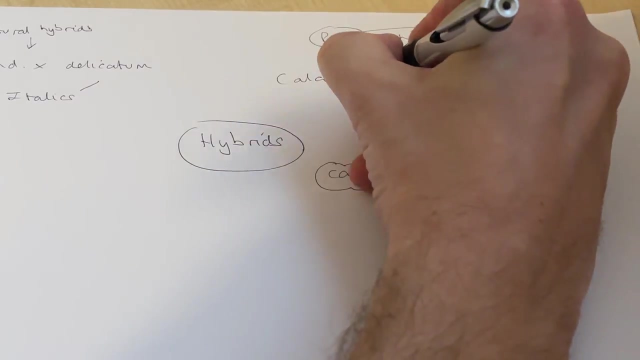 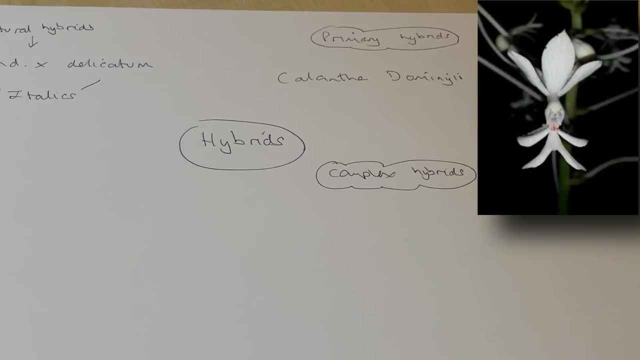 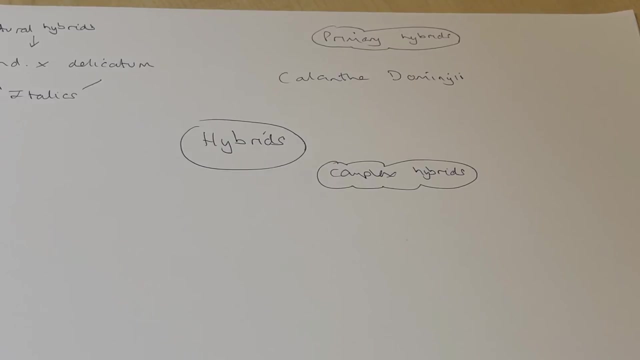 So I'm going to use one of the examples that I've got from one of those Websites I mentioned earlier. So we're talking about something called a Calanthe dominiae. Now, it's not an orchid I've ever heard of before, but what we can do is point out some of the ways that this should be written to show you straight away that this is a hybrid and not a species. 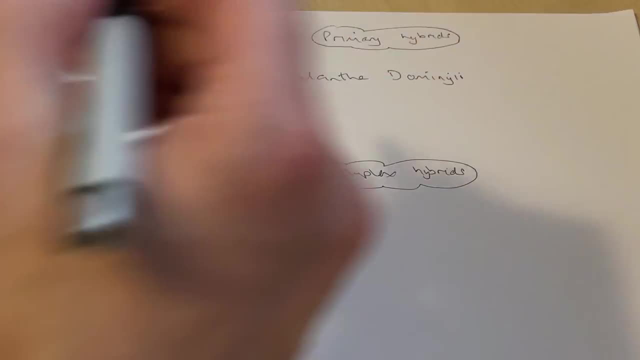 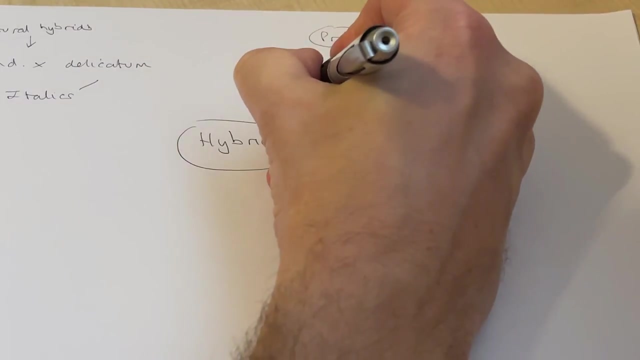 So the first thing to note is that the genus might be in italics. And again, this is where it becomes difficult, because I can't write It's in italics, so I can't actually show you. You can tell at a glance if it's been written correctly. 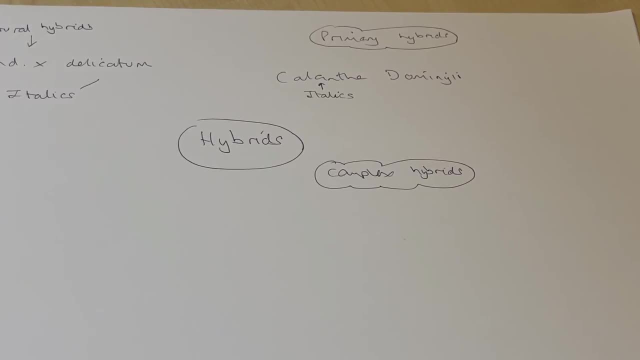 I have noticed on the RHS website they're all written correctly, which is really nice to see. So Calanthe is in italics. The following word, the second word in the binomial name, isn't in italics and it has a capital letter. 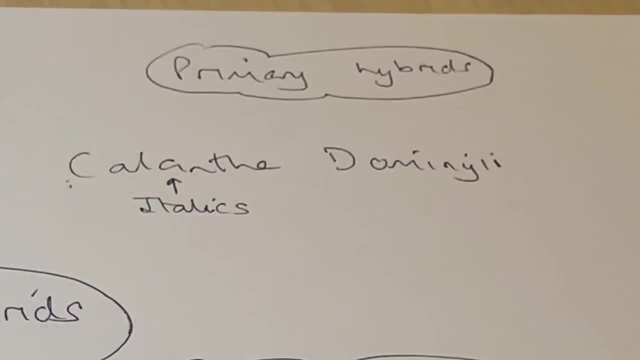 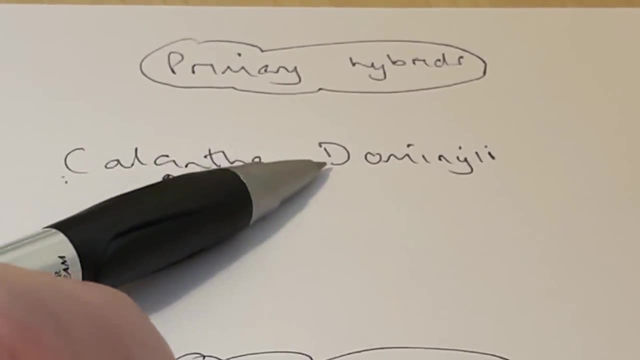 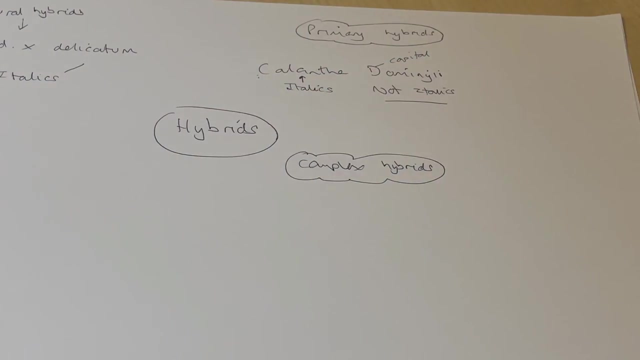 Both have a capital letter, in fact, so that doesn't change That one is a capital letter, Regardless whether it's a hybrid or a species. whereas in a hybrid that second word is not in italics, The letter of that word, the first letter, is capitalised. 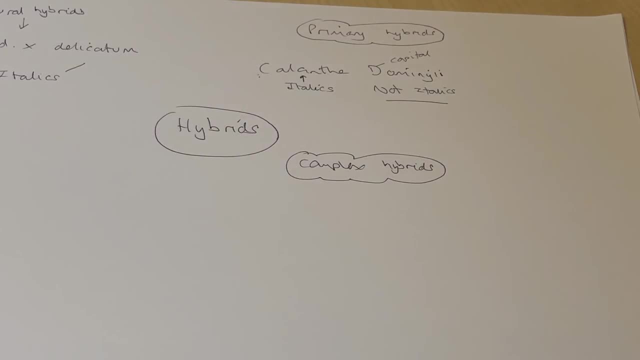 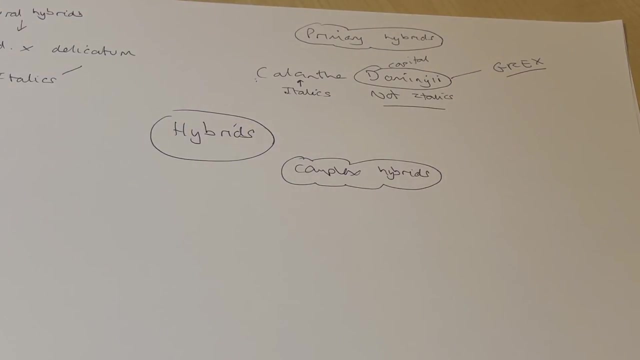 So this is made by crossing two species of Calanthe. So this second word is a special word given to it, called the grex. So that's worth remembering because you'll see, when you come to these various websites that help you with this, that they ask for the grex. 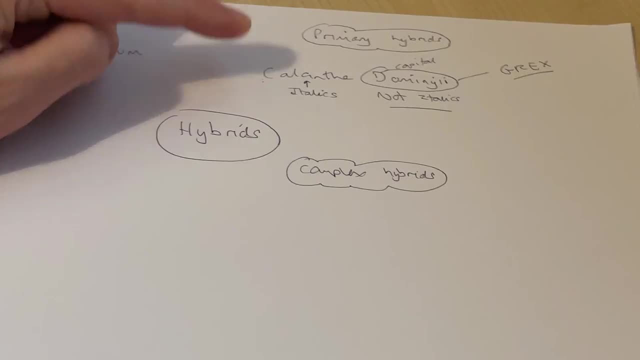 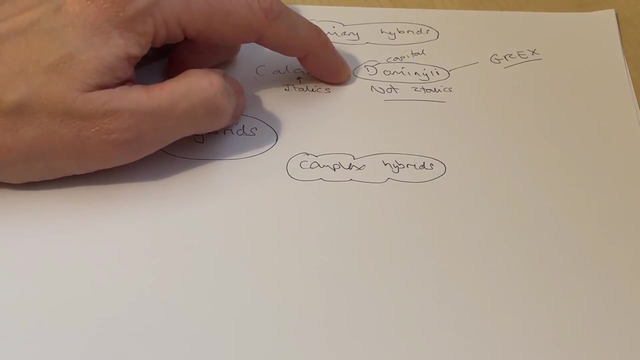 They don't actually ask for the genus. They always ask for the grex. Not quite sure why, but then you'll find that when they give you the list of the results, there can be many, many different genus that have the same grex. 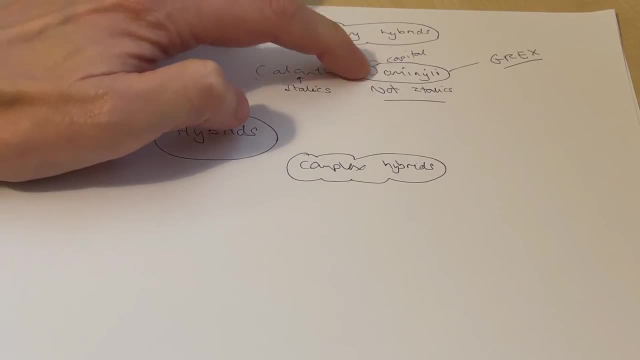 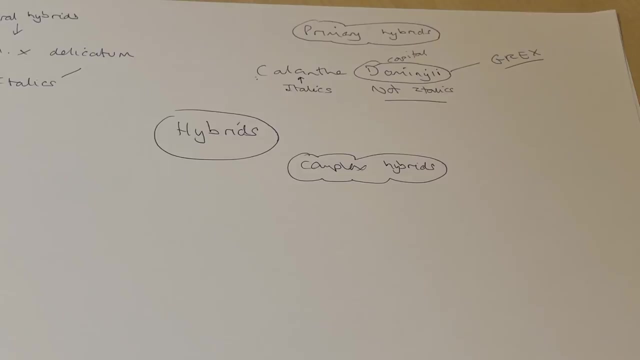 So if it's combined with the genus, then there can only be one grex that goes with that genus, And then all the progeny of that particular plant will have the same grex. And now we're getting to the bit where it becomes even more complicated. 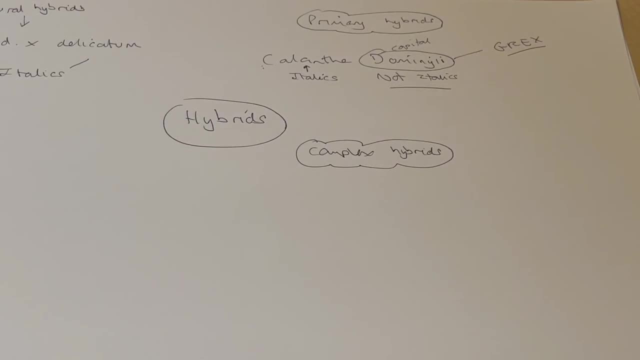 because the complex hybrids are when we cross either two or more hybrids or a hybrid and a species. So whenever there's a hybrid involved in the crossing of orchids, then it's going to be a complex hybrid And I've got many examples of that. 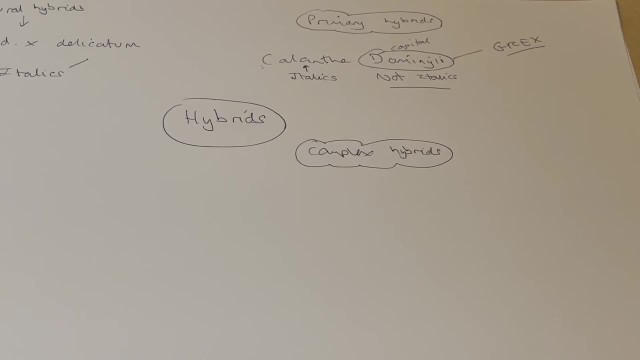 And, in actual fact, when I go to the orchid societies and I've always wondered why- I don't know whether this has anything to do with it, but a lot of the guys that have been growing orchids for years- they go through like a journey with it. And eventually a lot of them seem to kind of settle on either doing primary hybrids or natural hybrids or species plants. Some of them just only do species. There are very few of them that get into the complex hybrids. Now, the complex hybrids are supposedly easier to grow. because the reason that we create these hybrids in the first place is because there's something about that particular hybrid that is better than what we had originally, Whether it's a bigger flower, a bloom that lasts longer, or it can cope with more conditions, and so on. So I suppose if you're an orchid purist, it may be that you consider those to be not for a real orchid lover, And only the real orchid lovers get involved with just the species. That's just my theory. I don't know. 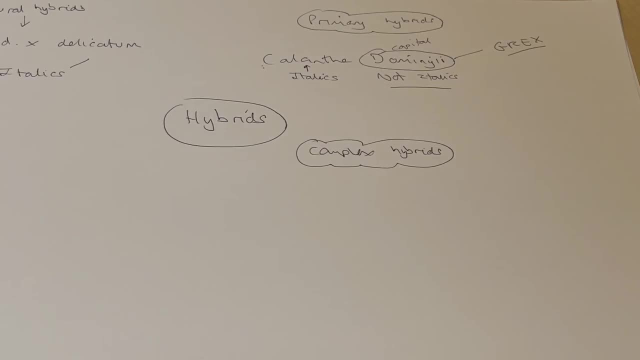 Maybe somebody can comment on that and see why I may eventually land the myself as time goes on. So these complex hybrids, I guess, are like frankenplants, aren't they? They're Frankenstein's monsters of a plant. They couldn't possibly exist if it wasn't for people tinkering around with pollen and fruits and so on. 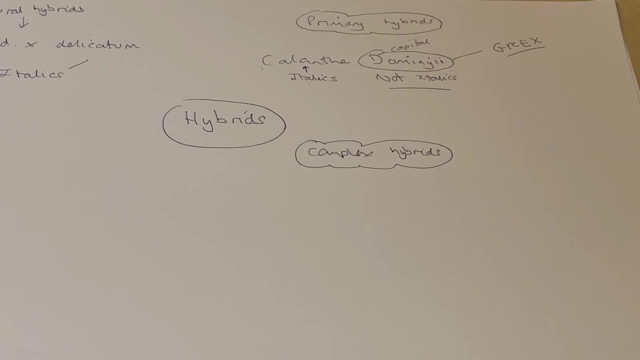 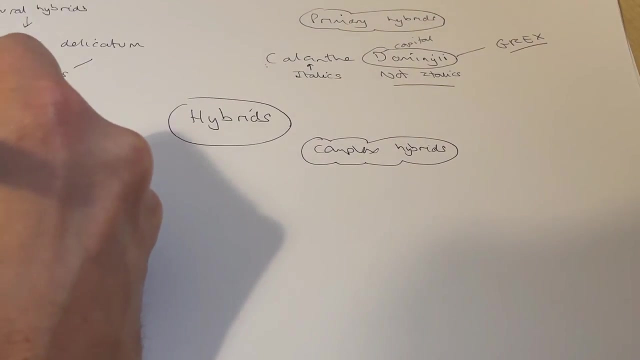 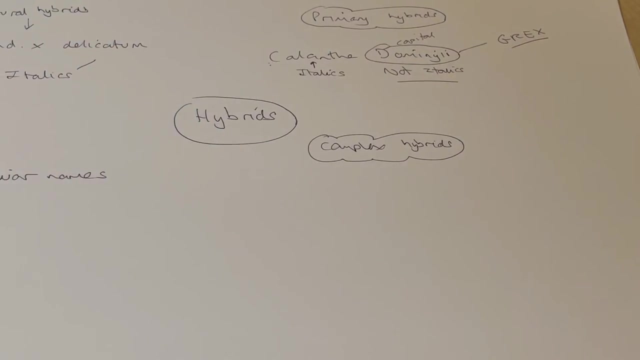 and trying to come up with something a little different. So the complex hybrid rules will follow the same rule as the primary hybrid, except we now begin to add things in like cultivar names. Now I've always used cultivar and hybrid kind of interchangeably. 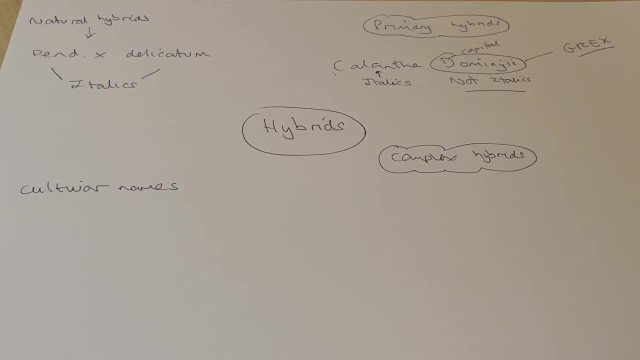 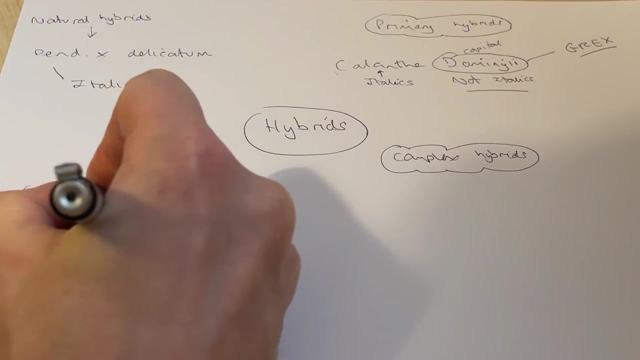 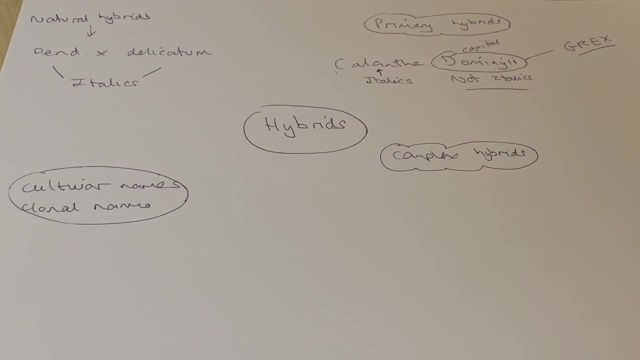 and they're not actually the same thing. So sometimes- and to confuse it even more, sometimes it's also known as the clonal name or just a clone. So those two things are the same as far as I can tell. So a cultivar name or a clonal name is a special name that's given to either a hybrid or a species. 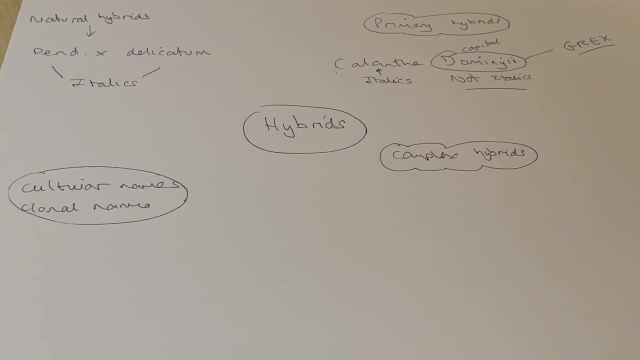 It could be in either. So a cultivar name could be a species or it could be a hybrid. worth pointing that out a couple of times. The way it's shown is it's just a name that follows the binomial names, but it's in quotation marks. 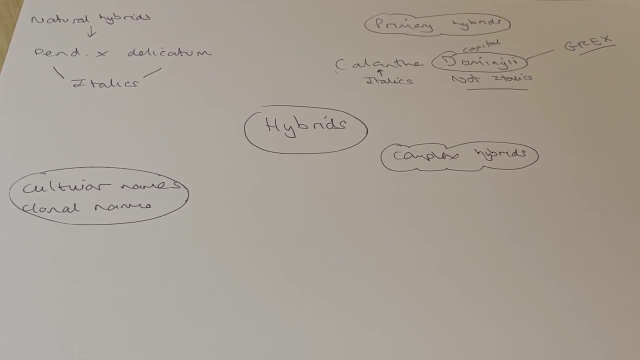 So these are names, special names given to these plants if they have something outstanding about them, or maybe they've won an award So they may be particularly easy to grow. They might they might have some specific characteristic that means that they're going to be awarded this special cultivar name. 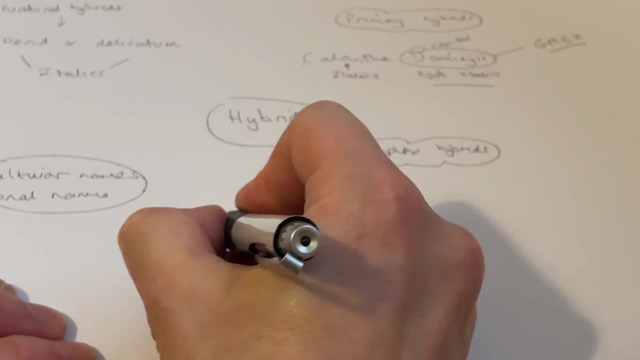 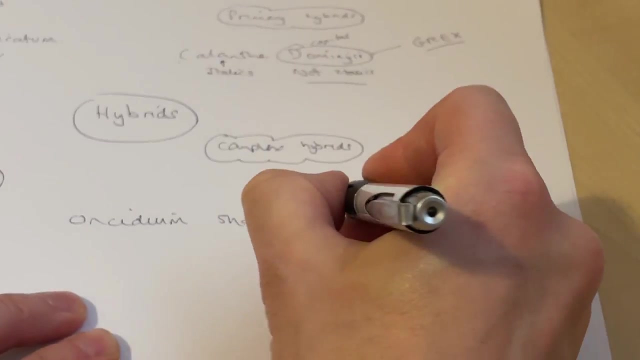 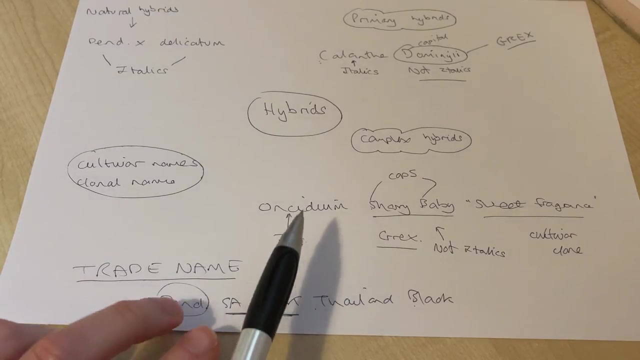 So, for example, here's one that I have and you might be familiar with, So an Oncidium sherry, baby sweet fragrance. Okay, just to speed things up a bit, I've already written it out. So we've got Oncidium sherry, baby sweet fragrance. 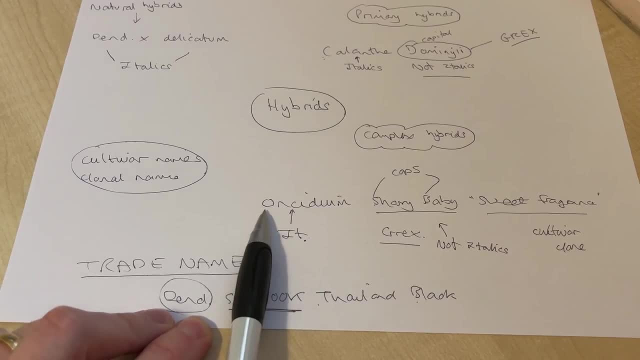 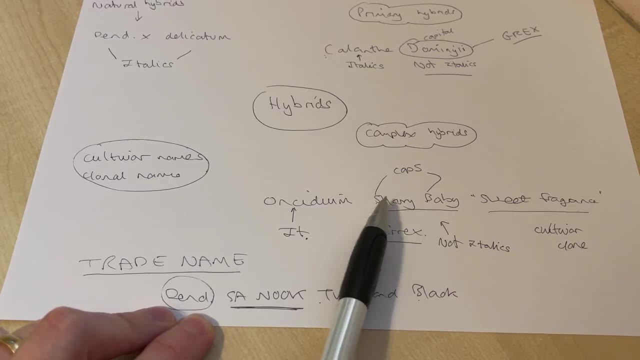 So this is a complex hybrid. So Oncidium, capital letter, should be written in italics straight away. You should see that sherry baby isn't written in italics and they both begin with a capital letter. So that's in normal Roman times or times, Roman font. 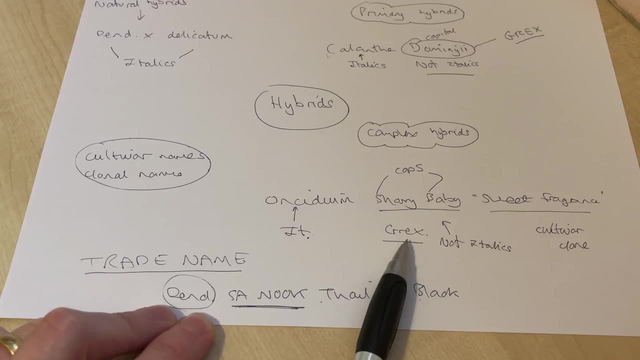 That's your Grex. If you're going to do a search on this particular cultivar, then that's what you need to use to search, And this one has been awarded as a clonal name or a cultivar name of sweet fragrance. 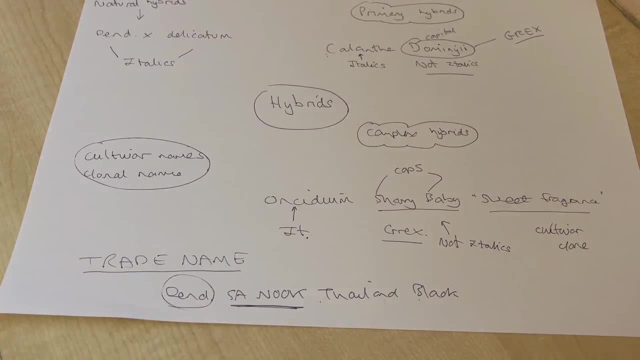 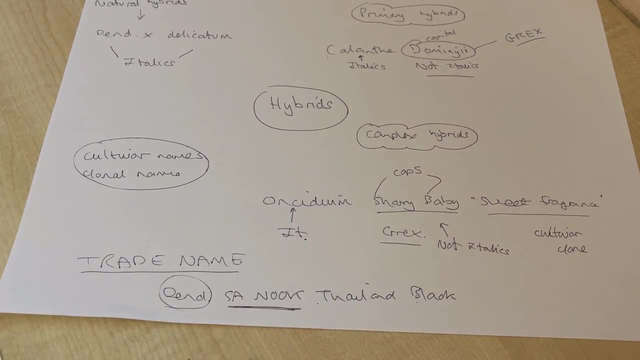 And that goes in quotation marks to either side. So that's the general form that most of these complex hybrids will follow. You will find variations on it, For example trade names. So for a trade name, something like a Dendrobium. 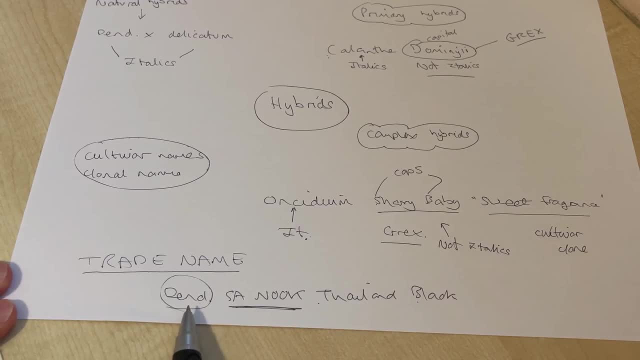 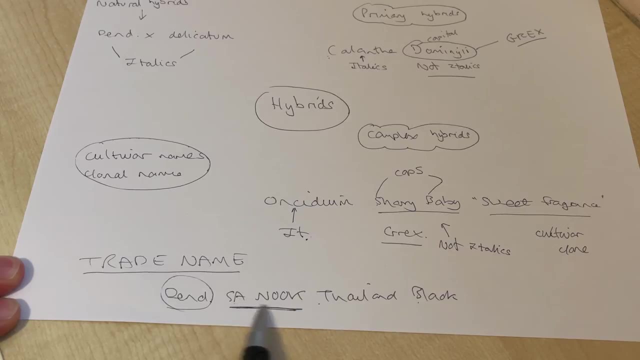 most of us are familiar with the Sarnuk hybrids, So if it's a trade name might not be Sarnuk, it might be another trade name. that should be in capital letters and not in italics. Dendrobium will still be written in italics. 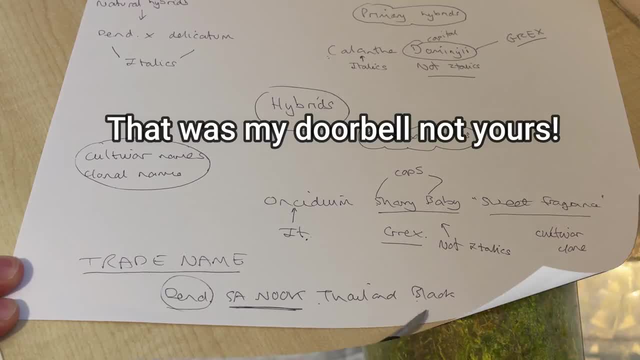 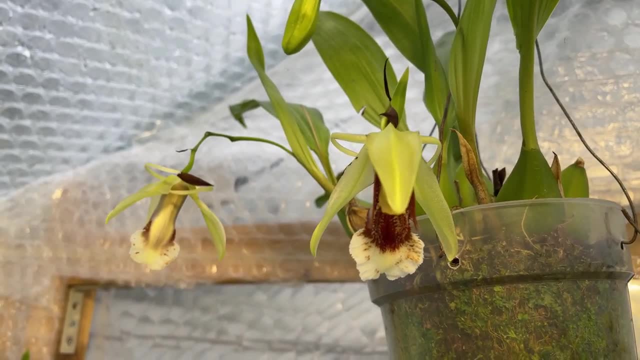 Tarn and Black. that's the Grex And that won't be written in italics. So just to finish things off here, rather than simply give you the information and not do any practice, what I'm going to do is go through a few of my labels here on the screen. 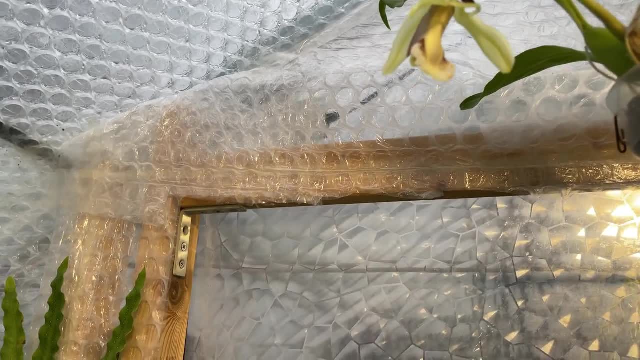 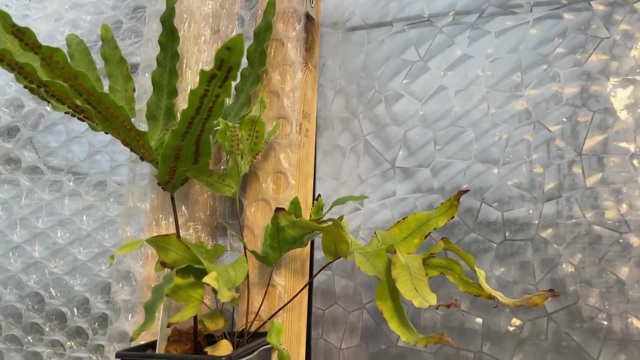 while we're looking at a few sweeping shots of the greenhouse that I took quite recently And we can have a practice and see if we've all kind of got it in our heads. OK, the first one that we're going to look at is Mastivalia snowbird. 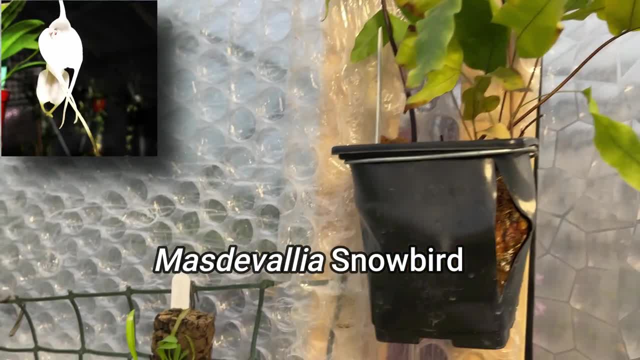 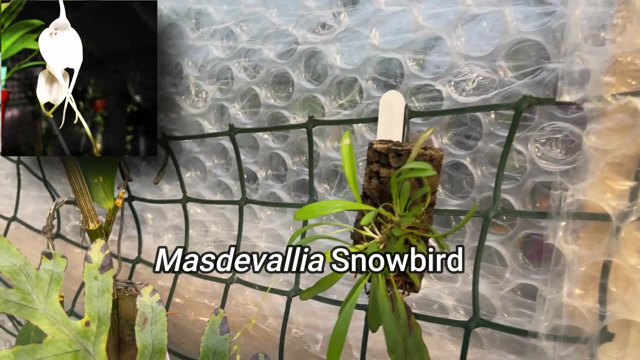 which I have in the greenhouse. So the first word begins with a capital letter. That's the genus, And it's in italics. The second word, because it's not in italics and it begins with a capital letter. 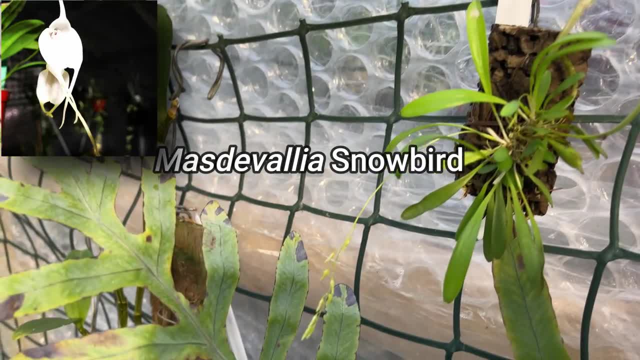 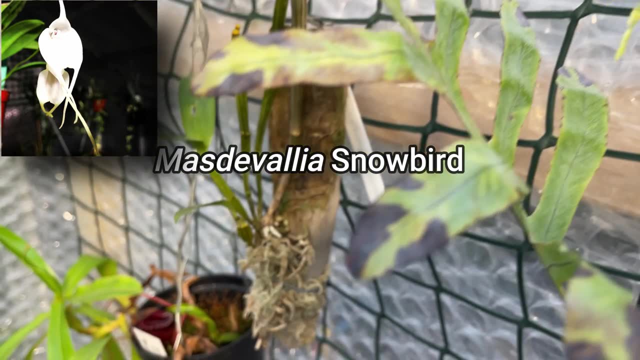 that tells you straight away that this is going to be a hybrid. So snowbird is the Grex And this is a hybrid between two Mastivalias. Now we don't know whether it's a primary cross. What we'd have to do is look up the Grex snowbird. 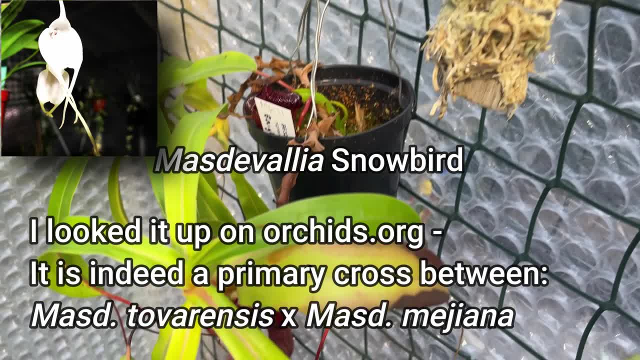 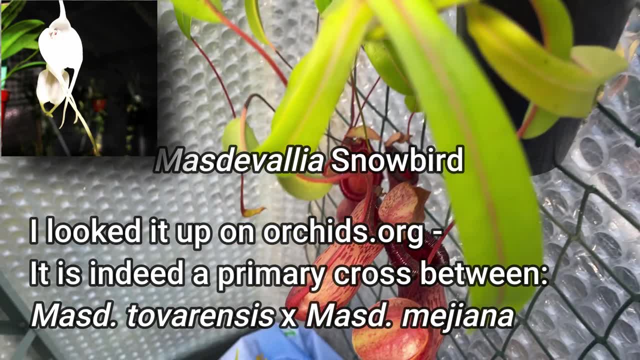 and see whether the two Mastivalias that's been crossed, to see whether they are both species. If they're both species, then it's a primary cross. If at least one of them isn't, then it's not a primary cross. 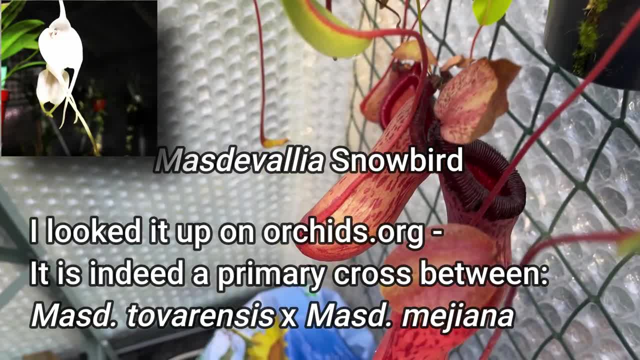 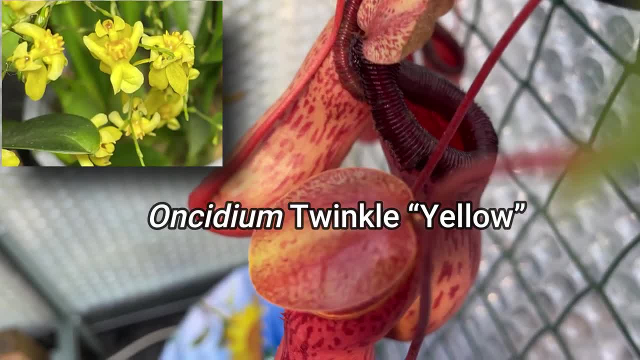 It's just a complex hybrid. So the next one we're going to look at is Oncidium twinkle yellow. So this again, because the first word begins with a capital letter and it's in italics and the rest of it isn't. 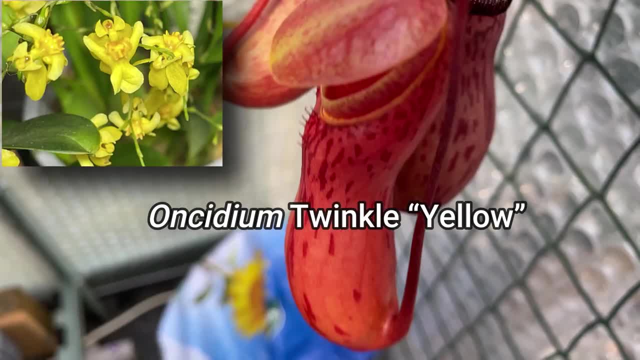 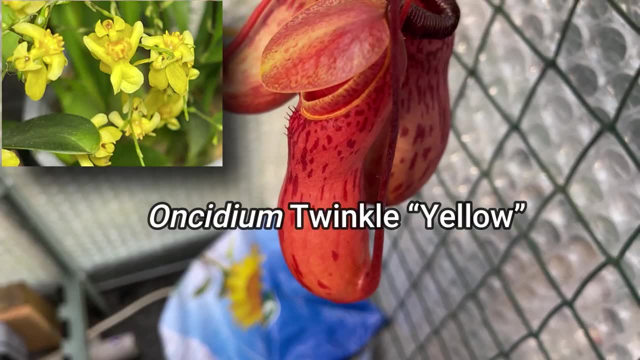 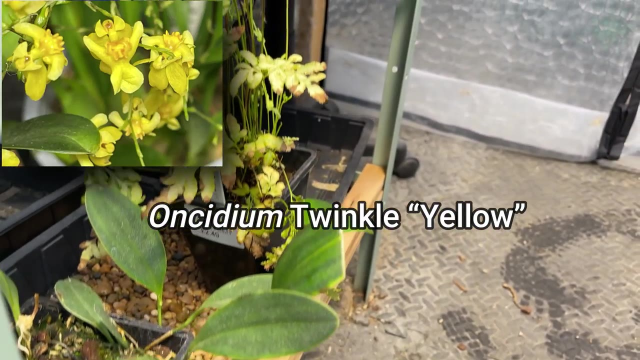 that tells you that this is a complex hybrid. Twinkle is the Grex, And this has also been awarded a cultivar name of yellow, And that's the knot in italics and in quotation marks. So this is actually a primary hybrid. 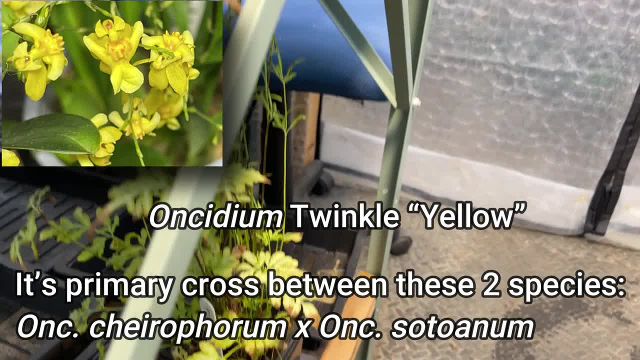 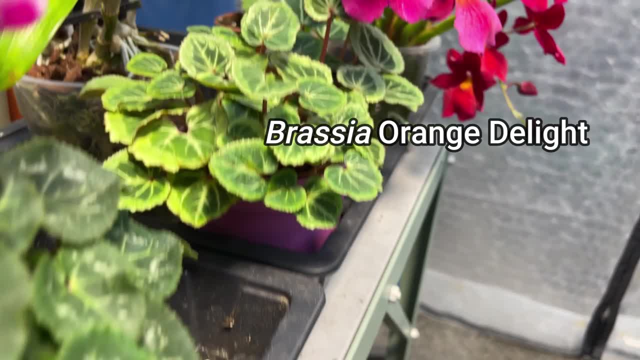 which means it's a cross between two species. So this one is a primary cross. I'm trying to give you an example of most of the different possibilities. So let's look at Brassia orange delight. So this is a hybrid between two Brassias. 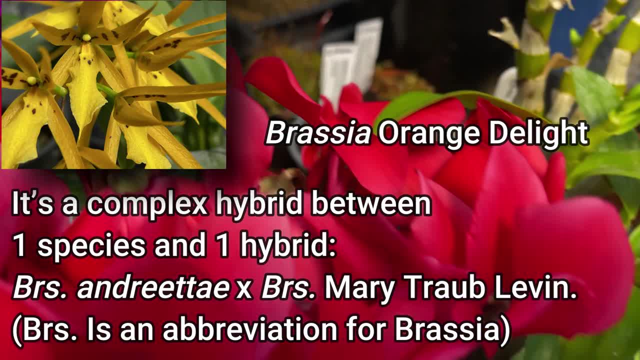 So Brassia is the genus that's in italics, Orange delight isn't in italics and it begins with capital letter. So that tells you it's going to be a hybrid. Again, I'd need to do a little bit more research.